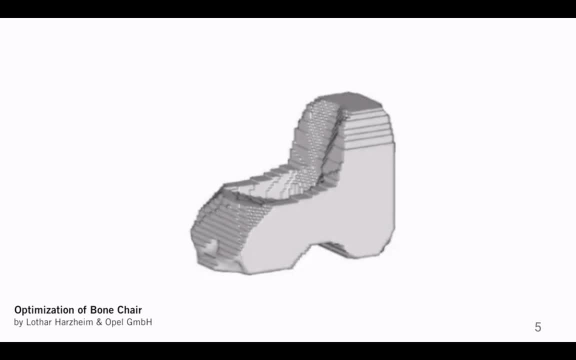 Let's have a look how this shape evolves during the iterative optimization process. It starts from this solid block, And here we could observe the seat and the back, And these two parts are not allowed to be changed during the optimization. And on the ground there are three points fixed. 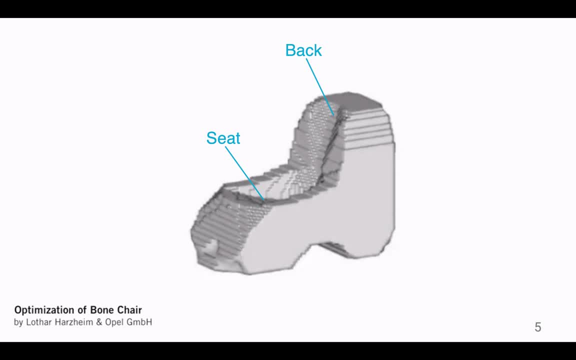 Indicating where the necks will grow from. So let's have a look at this animation. This optimization process is an iterative process. During these iterations, the material that is not relevant for this mechanical load. the material that is not relevant for this mechanical load. 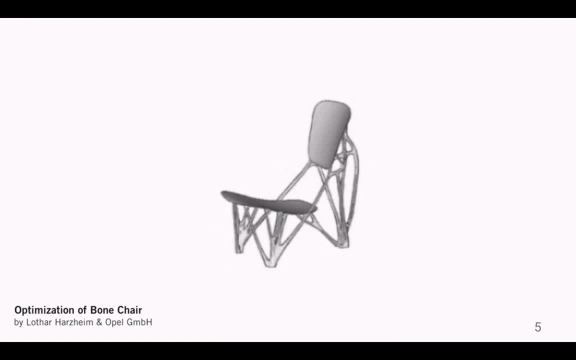 is automatically removed. This process is very similar to how our bone reacts to mechanical load. Because of this natural adaptation process, what remains is a very elegant structure to support the mechanical load in the best way. This skeleton looks visually comparable to the bone. 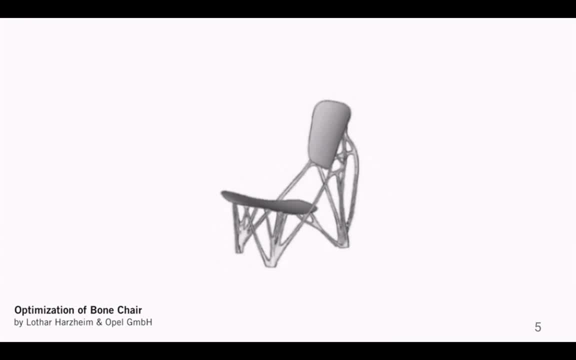 and also the principle behind the design of this chair is similar to the bone adaptation and this gives the name: the bone chair. We have a design and each design. we would consider fabrication Back in 2006, 3D printing is not as mature as of today. 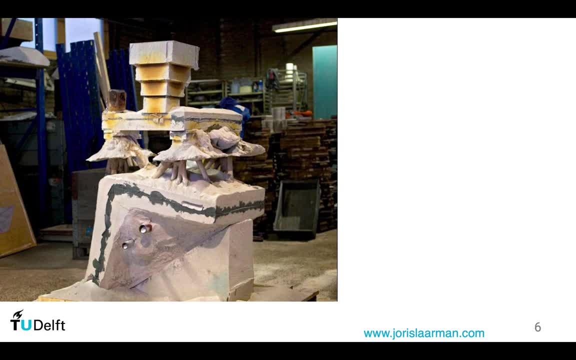 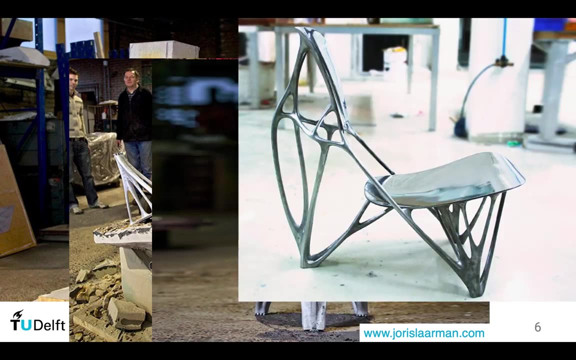 It is called rapid prototyping. What the designers did was to fabricate a mold by using rapid prototyping. It composed of multiple pieces. By casting aluminum into the mold, they eventually get a polished design, as shown here. So this is an iconic design of topology optimization. 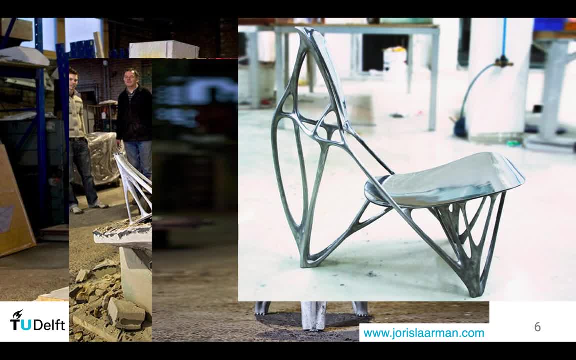 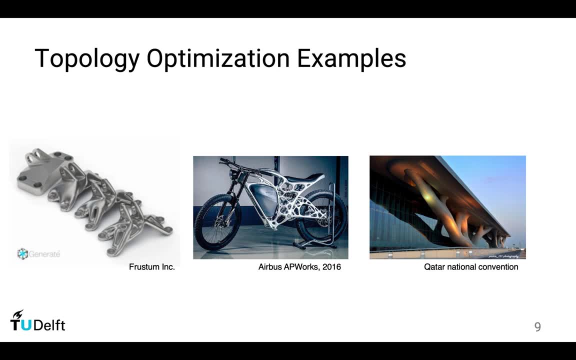 It is exhibited at multiple industrial design museums around the world. The chair is just one of the examples of topology optimization. Topology optimization is most relevant for aerospace and engineering. Topology optimization is most relevant for aerospace and engineering. Topology optimization is most relevant for aerospace and automotive industry. 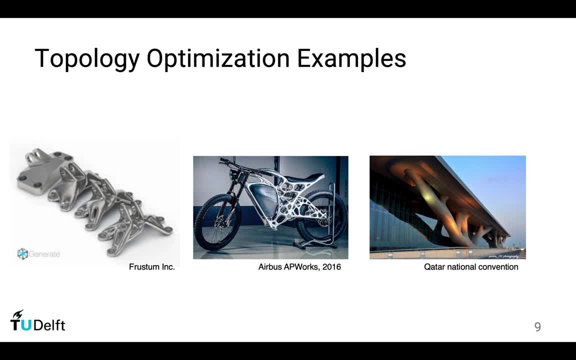 Topology optimization is most relevant for aerospace and automotive industry, And there people strive to reduce the weight of mechanical parts. For instance, on the left-hand side you see a bracket in an airplane. By using topology optimization, the mechanical weight is reduced significantly. 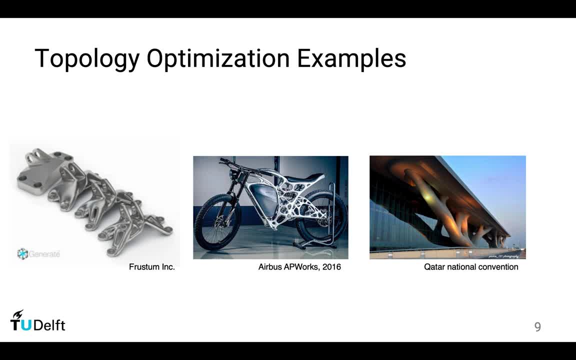 while not sacrificing the mechanical performance. In the middle it shows topology optimization applied to design motorcycle frames. In the middle it shows topology optimization applied to design motorcycle frames. It looks elegant, It is fabricated by 3D printing And on the right-hand side. 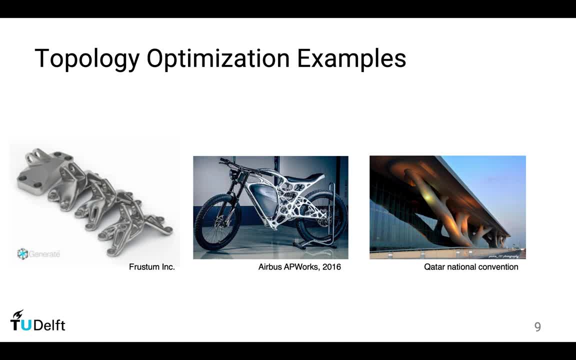 it is Qatar Convention Center. Topology optimization creates beautiful organic shapes And this is very much appreciated in art and in architecture, And that's the reason people apply topology optimization to design support structures for Qatar Convention Center, shown on the right-hand side. 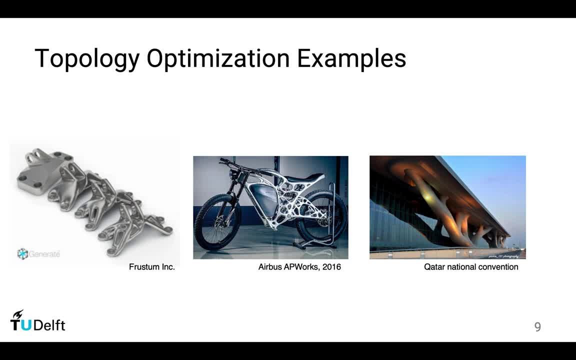 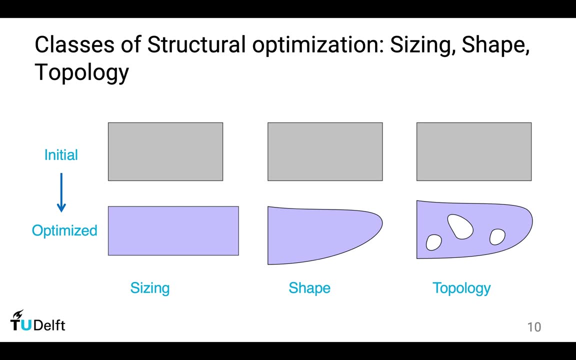 It is a giant structure. It is a giant structure. It has a length of about 260 meters and a height of 30 meters. Talking about topology optimization, we would like to distinguish other optimization classes. Normally we distinguish between sizing, shape optimization. 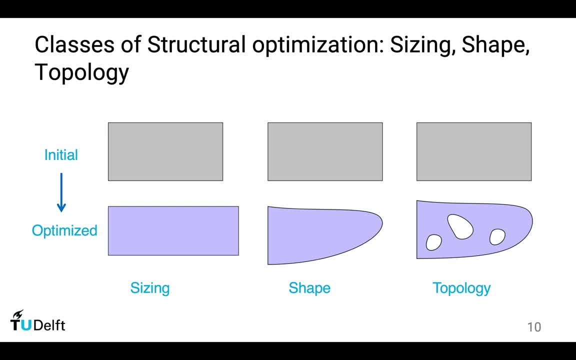 and topology optimization. Let's say we have a rectangular structure, We have a component, We want to optimize it for some purpose. You could optimize the dimension, For instance. you make it longer, You make it shorter, And this is called sizing. 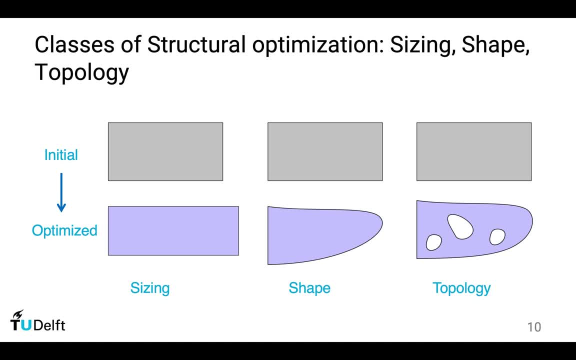 So you modify the size of the component Relatively. you can modify the outer geometry as shown in the middle, So you modify the boundary and make it curved, And this is called shape optimization. Topology optimization is different from sizing and shape optimization. 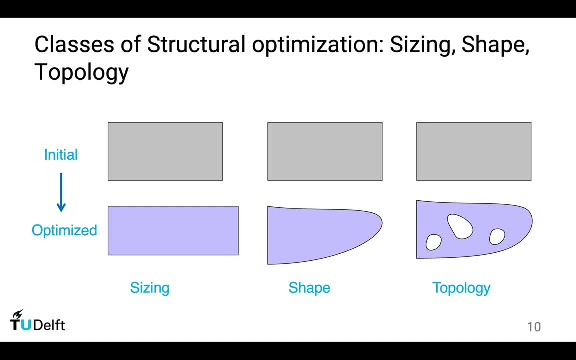 mostly on the aspect that the topology is modified On the right hand side with topology optimization, for instance, after optimization you get three holes in the geometry. The topology in 2D basically considers whether how many holes you have in a domain. 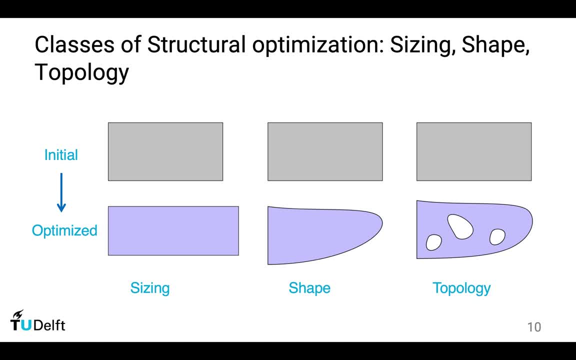 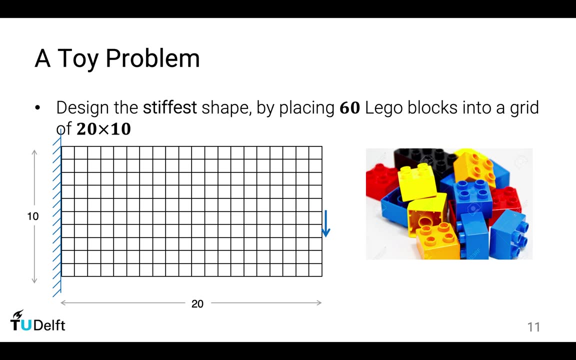 So in this case the topology is changed And to differentiate from sizing and shape optimization, we call it topology optimization. To explain the principles behind topology optimization, I would like to introduce this new, this simple toy problem. Almost everybody has played with negative blocks. 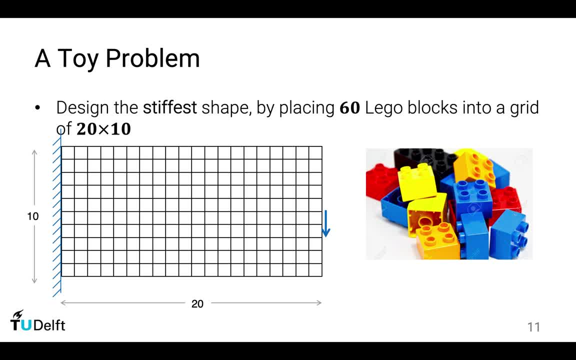 Normally, we are given a limited amount of resources and we want to make the best use of it. Consider: we want to build a structure in a design domain which has a dimension: 10 by 20.. So if we want to build a solid structure, 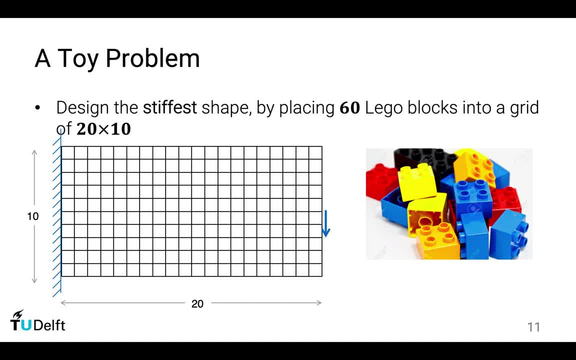 we need 200 Lego blocks And we want to find a structure such that when a force is applied on the right hand side, in the middle, downwards, we want to find a structure that has the minimum amount of deformation, Or in other words, we want to find the stiffest structure. 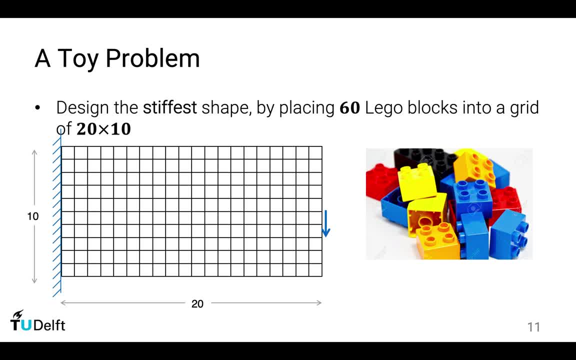 So if we want to build a structure, we have 200 blocks, That's very easy. We just make the entire structure solid. But now we don't have as many as we want. Suppose we have only 60. We have to place these 60 blocks in a very clever way. 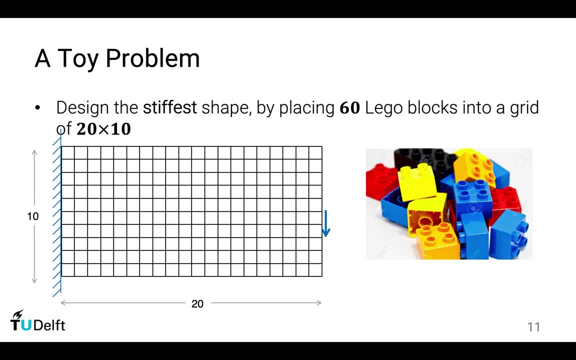 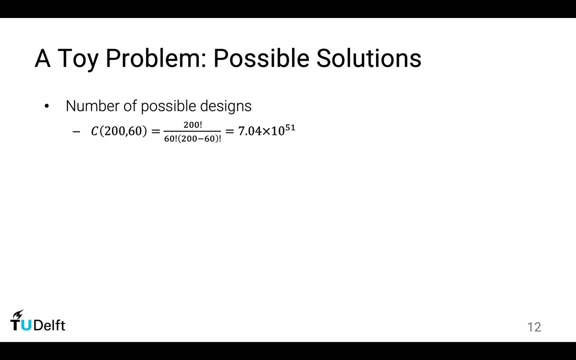 such that when a force is applied, the deformation is small or the stiffness is very high. And this is what we want to find out. So we have 60 blocks, We place it within 200 empty places. By calculation, we can find out. 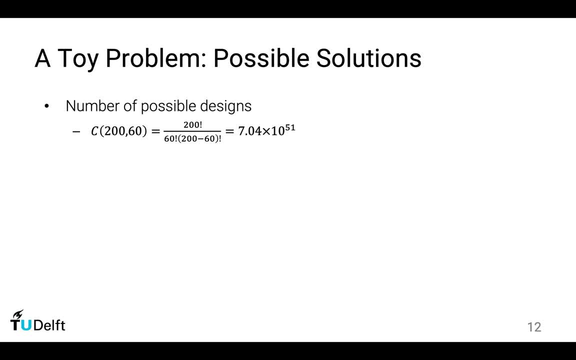 we have 10 to the power of 51 possible solutions. This is a huge number. In China, when we talk about a big number, a countless number, we say it's just like the stars in the universe. The stars in the universe by estimation. the number is about 10 to the power of 24, which is far less than the possibilities here. In fact, I have just checked the number of. if we consider the entire Earth, the mass would be composed of 10 to the power of 51 protons and neurons. 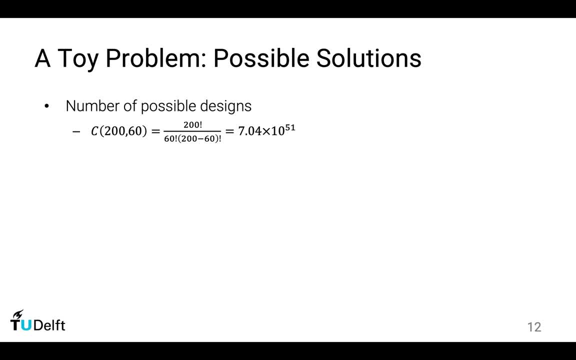 So all these atoms added together is 10 to the power of 51, which is the same size of our problem. This essentially tells us it is not possible to test every design, So I illustrate three possible solutions. Here we have 60 blocks. 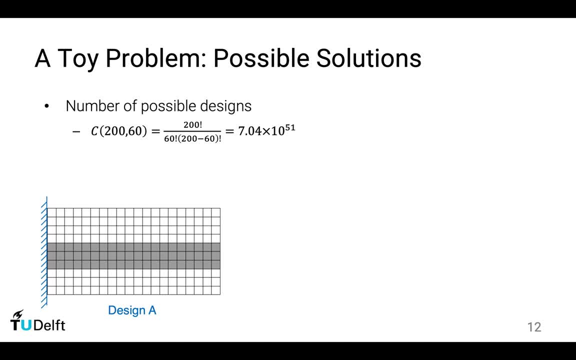 We divide it by 20, so we have three solid rows. Let's call it design A. You might think. on the left-hand side it is more important for supporting the node, so we place more blocks to the left. Let's call it design B. 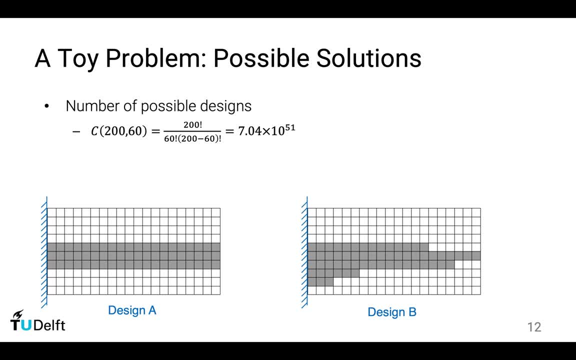 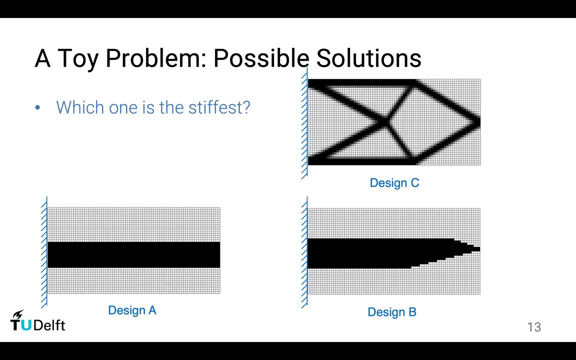 You might place it randomly by doing some tricks or black magic and you come up with design C And here we have three solid rows. If we increase the resolution to make a continuum structure, it looks something like this: Now think about it.